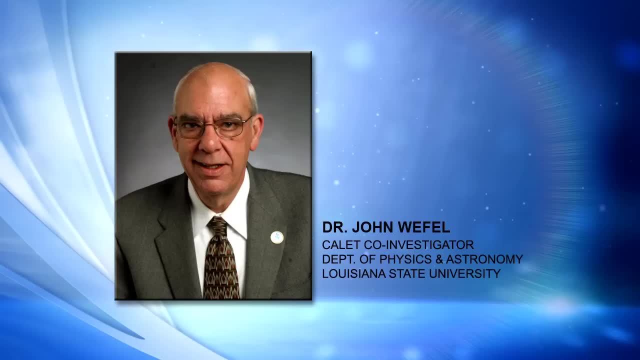 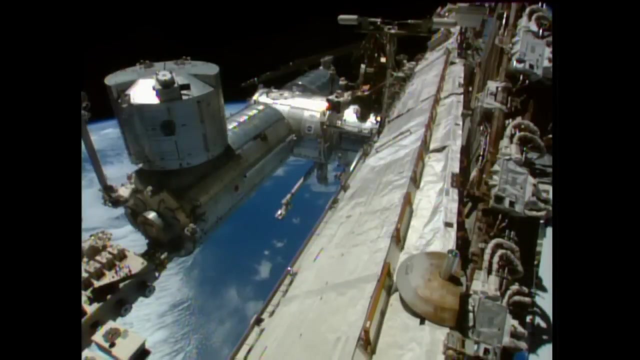 for example, the LHC at CERN. And what we're interested in is, A- how they do that and B- what material is being accelerated. Where did this stuff come from? And so to do that, what we want to do is we want to measure the composition. 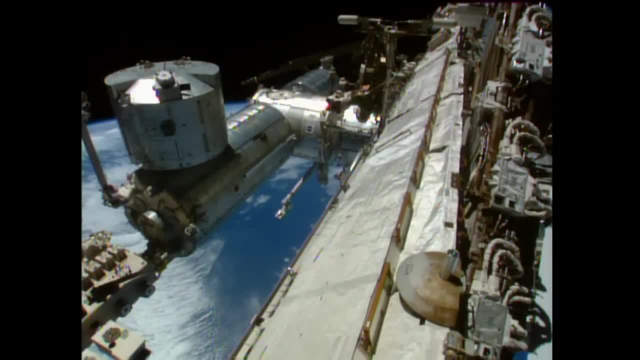 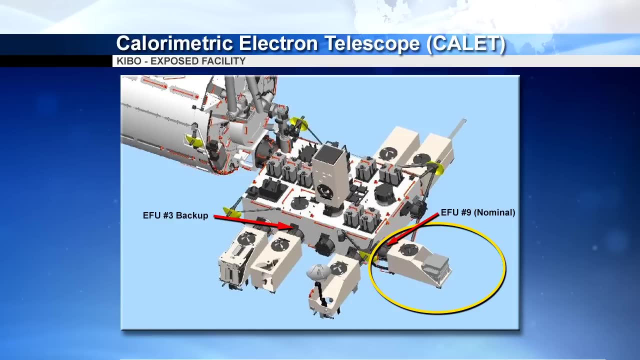 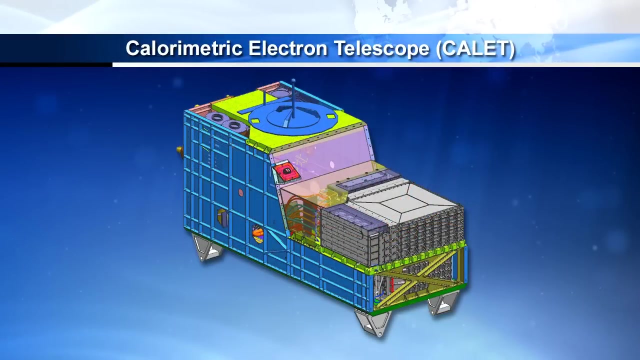 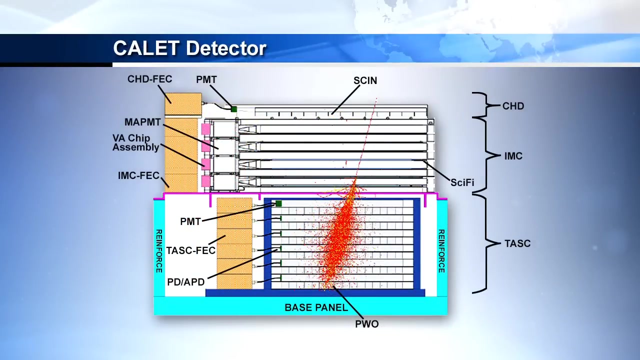 We want to know how many electrons are there, how many protons, how many helium, carbon, nitrogen, oxygen, iron, etc. to try to piece together this whole question of how nature works, how nature does this massive acceleration, how it ejects these particles that have been with us in our solar system for billions of years, based on the old meteorite measurements. 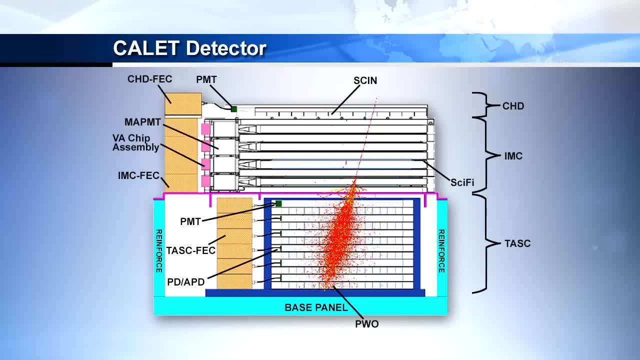 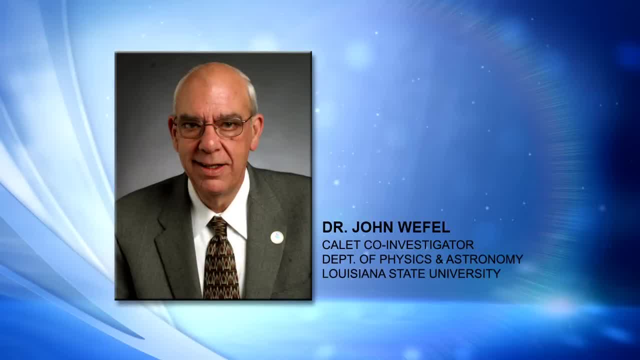 So they're a standard part of our environment. You're taking a census of what's out there. We're taking a census of what's out there, but we're trying to take it at higher energies than has ever been taken before, and that's the key. 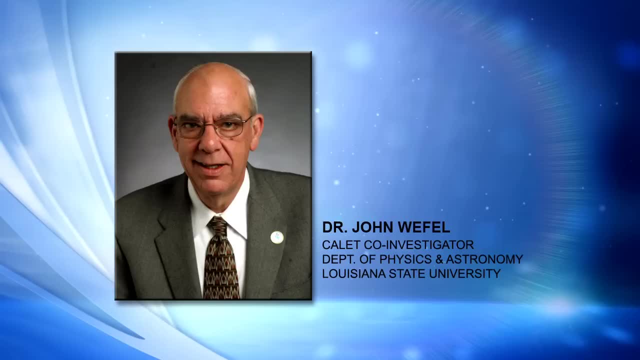 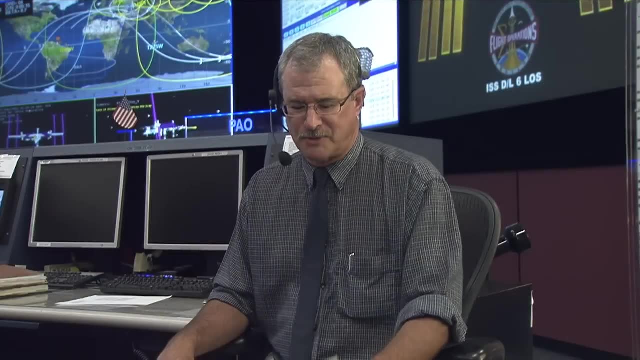 As you move to the higher and higher energy. that's where we're beginning to see now. that's where the action is starting to show up. Well, one of the stated goals here is that you're using this to address the existence of dark matter. 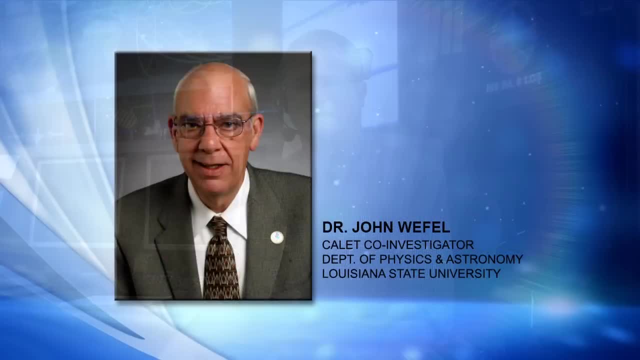 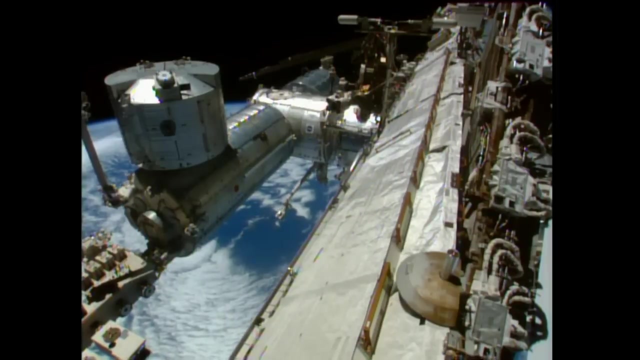 How does measuring cosmic rays help you do that? Well, the whole idea here is that if there are dark matter particles out there of one sort or another and they're their own antiparticles, so they annihilate with each other. when they do that, they turn into normal particles. 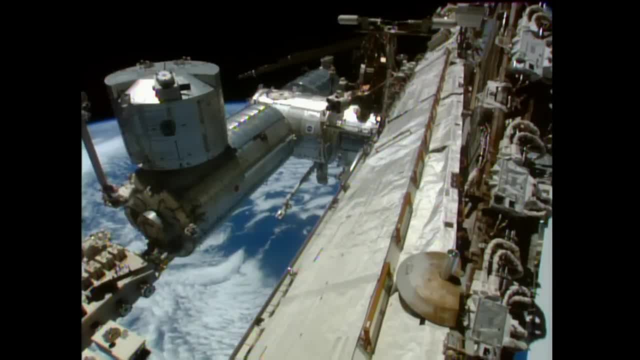 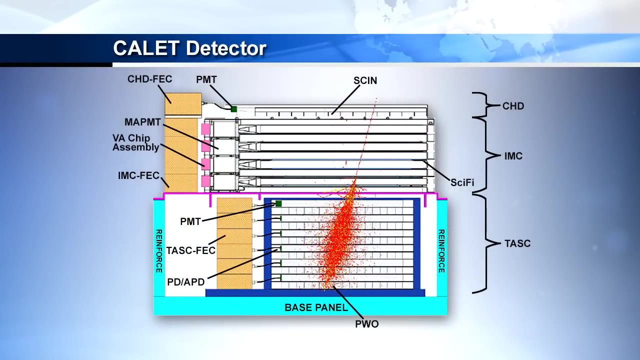 ie they turn into electron-positron pairs or they turn into proton-antiprotons or they turn into various kinds of W bosons, things like that. But when they do that, their mass energy, their rest mass, becomes their kinetic energy. 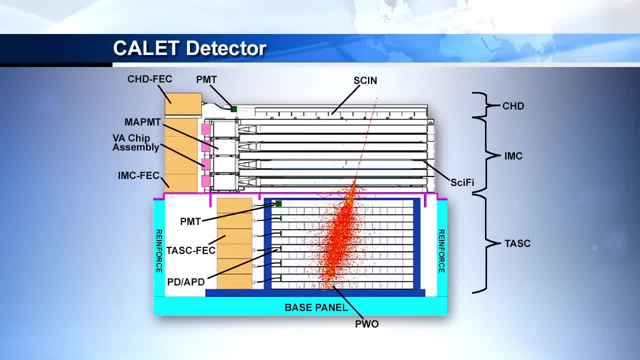 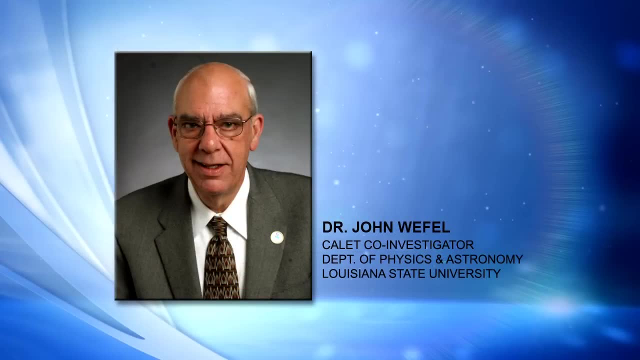 So they suddenly appear at these very high energies As a particle zipping around, just like the cosmic rays. so the idea is you may be able to find them within the cosmic ray beam. Now, to do that we have to look and see if we can find some kind of anomaly in the electron plus positron spectrum. 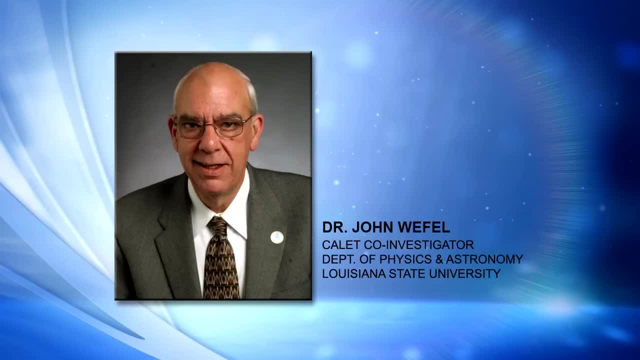 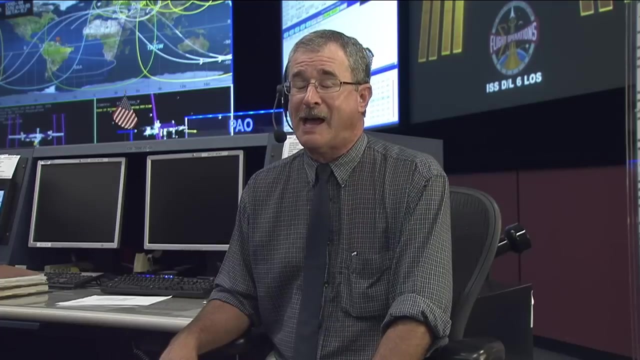 or we also have a capability to measure very high energy gamma rays. see if we can find a signature in the gamma ray region at these ultra-high energies. I also read that you're interested in finding what it says are nearby sources of high-energy cosmic rays. 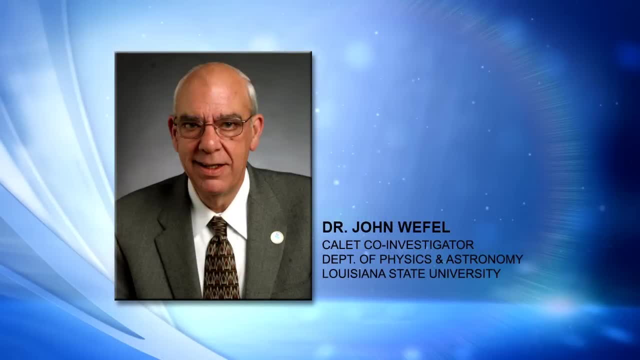 I mean, how close are you looking? Okay, well, nearby. has to be viewed in an astronomer's terms, if you will. What we're basically looking for is sources that are within about 1,000 parsecs of the solar system. 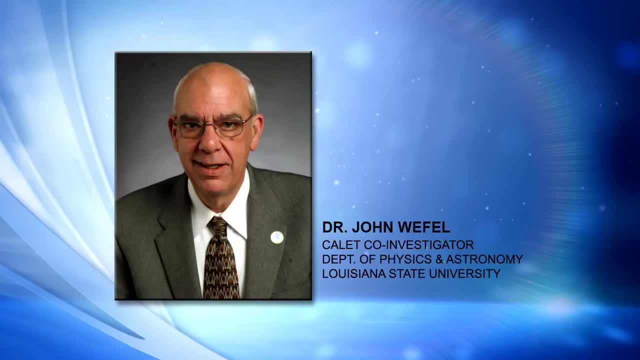 and are less than about 10 to the 5th years old, Less than about 100,000 years old. Why is that? Well, the reason is that electrons, unlike protons and other particles, they lose energy via inverse Compton and synchrotron processes. 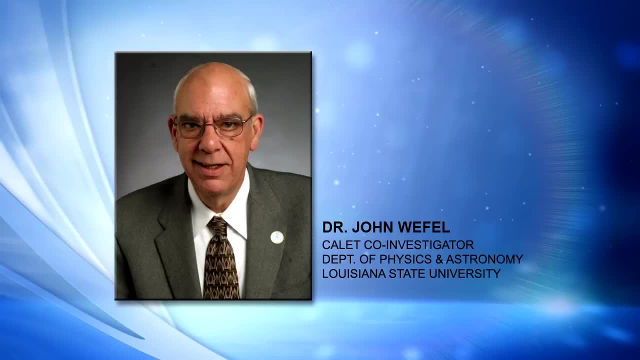 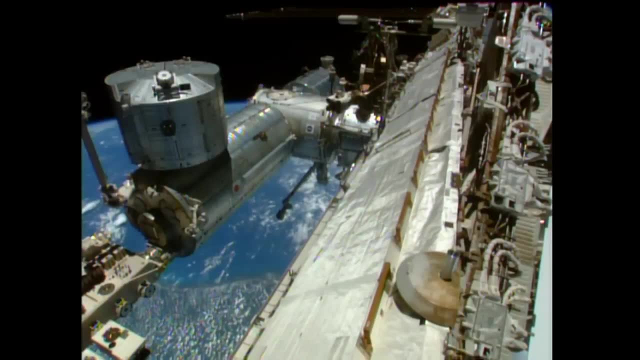 as they move through the galaxy, interacting with matter, photons and magnetic fields, And they lose energy at a phenomenal rate. What that means is that these very high energies, they can't travel very far before they're totally degraded. Thus anything we see has to be coming from somewhat relatively nearby. 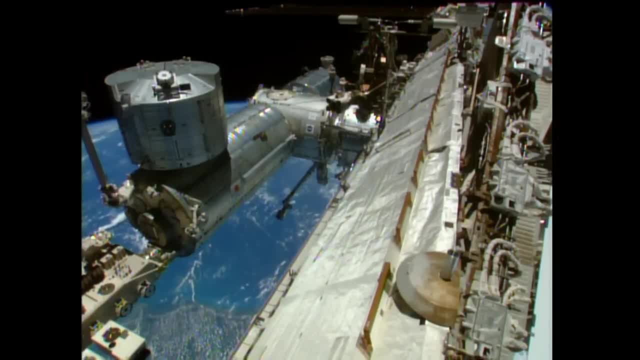 otherwise we'd just never get here from there. So in that sense, what you do is then you sit around and you say: well, what's out there, within a kiloparsec from us? And you find things like supernova remnants, monogens of supernova remnants. 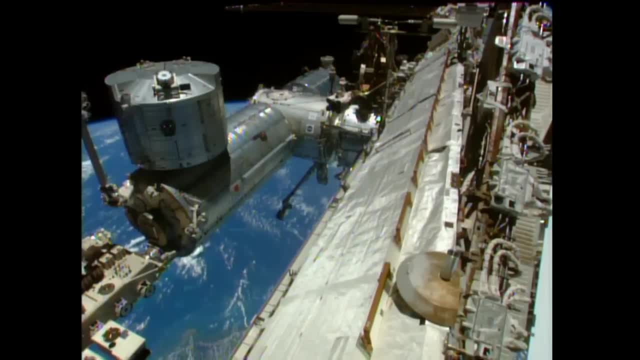 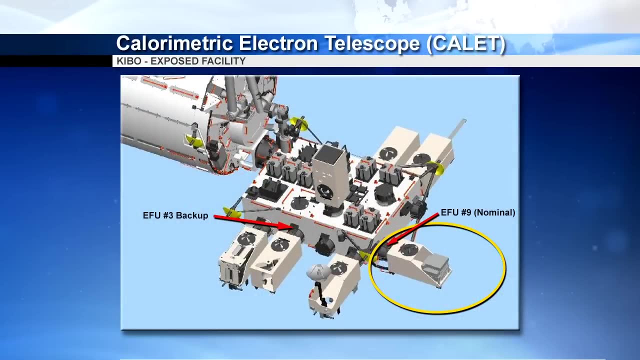 Cygnus loop, the Vela supernova remnant, And you say, well, could these be producing high-energy electrons? And so you go back to some of the theories and do some more calculations and you come out with yes, they could be. 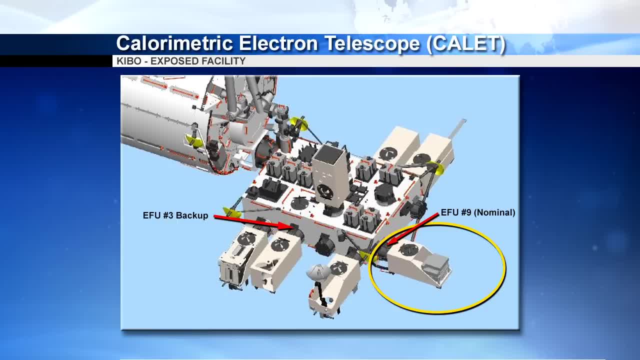 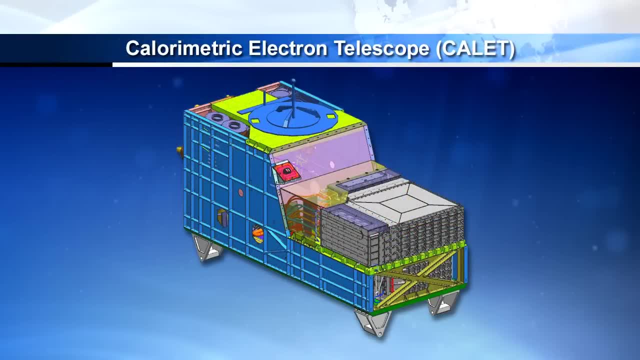 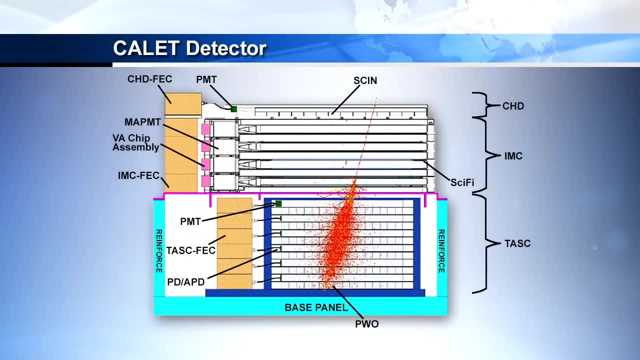 Maybe not, but they could be. So the idea being, if we can see one of these sources sticking up beyond, above the normal background of all the other electron-pyletrons that we're seeing, we would be able to actually pinpoint for the first time.